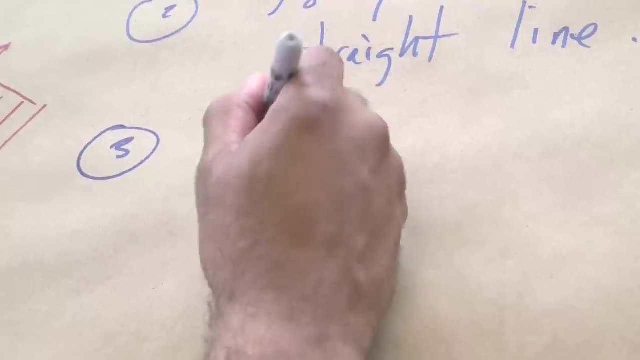 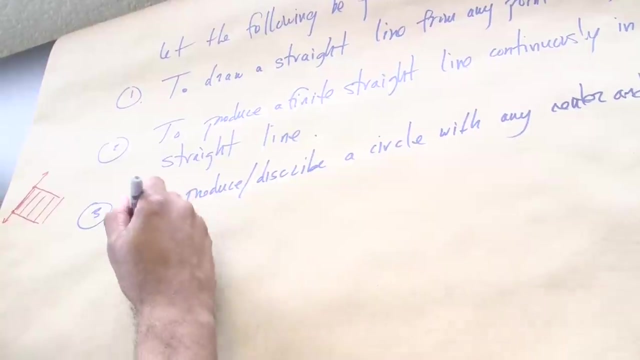 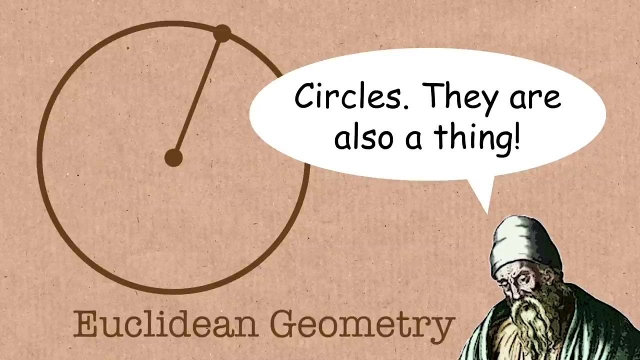 points and lines and we've created a plane. We can move to circles, To produce a circle with any center- that's a point- and any distance or radius. We've gone from points and lines and planes to now allowing some other objects to live in our world circles. The first three: 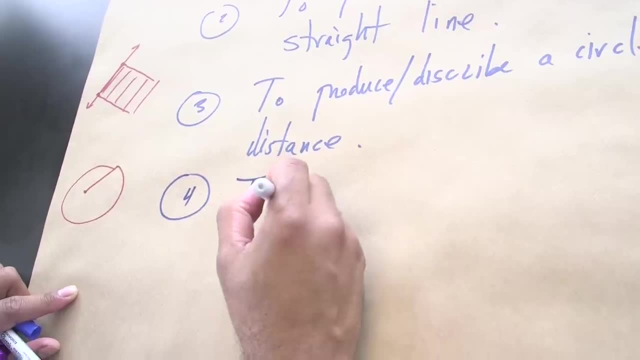 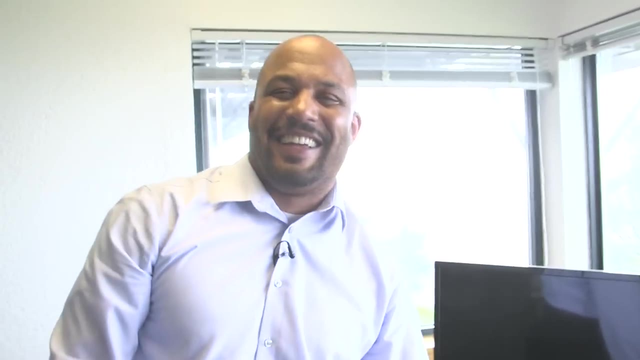 seem straightforward enough. Number four: things start to get slippery. Number four is that all right angles are equal to one another. Well, that's got to be the most obvious of all of them. Why do we even need to say that? What a right angle is requires definition, and you could actually start by defining what. 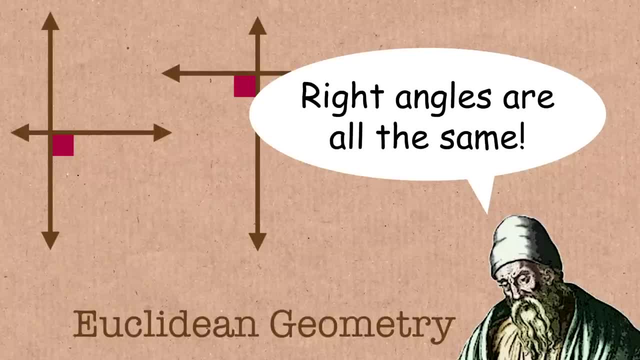 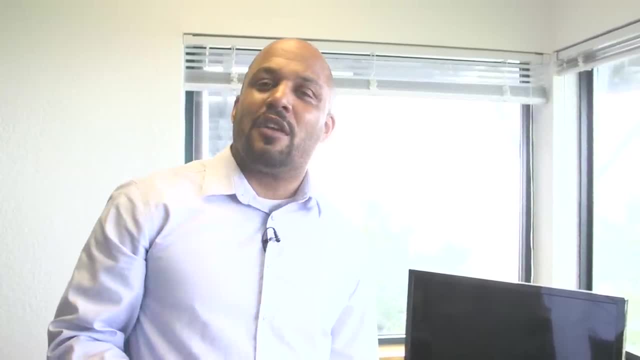 points and lines, and these basic objects are, But the notion of equality is more subtle, because do we mean equal in the sense of is, or this is exactly the same as that, or a notion of congruence? We've got four. Now we're coming to the fifth. This is the one that we should be paying attention. 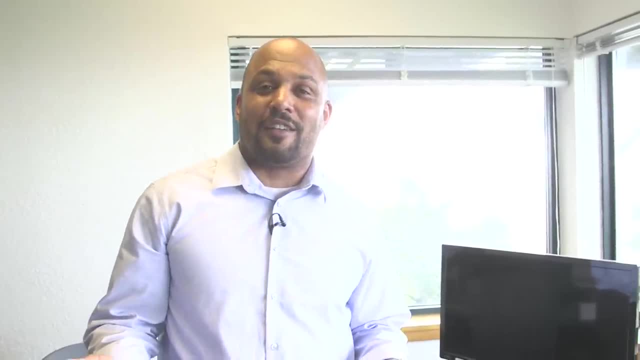 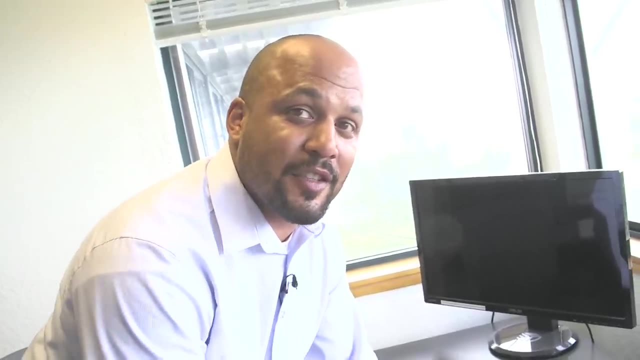 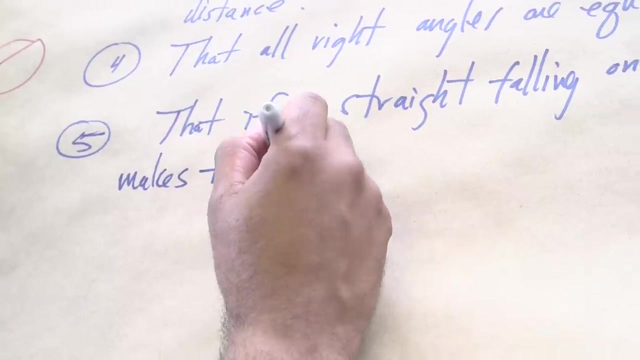 to. That's right. So here comes the fifth, The fifth possible. Let's write it down the way Euclid wrote it, and then we'll decide for ourselves what it means: That if a straight line falling on two straight lines makes their interior. 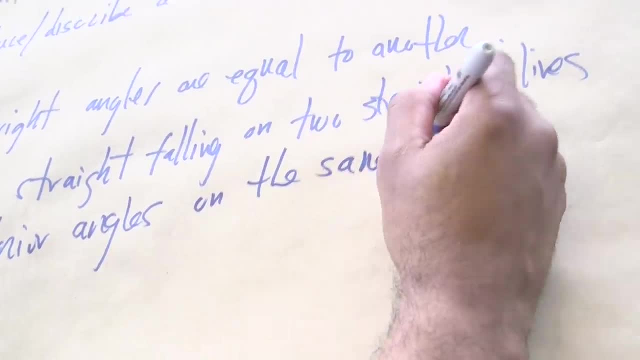 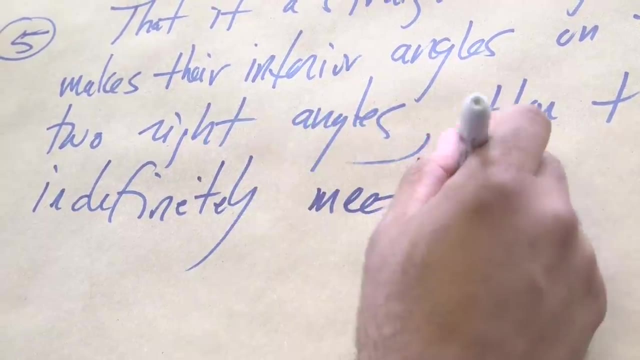 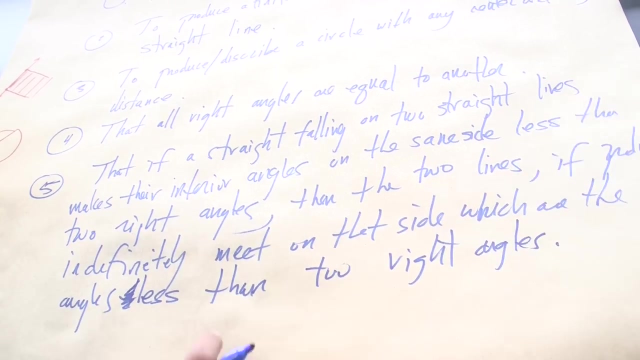 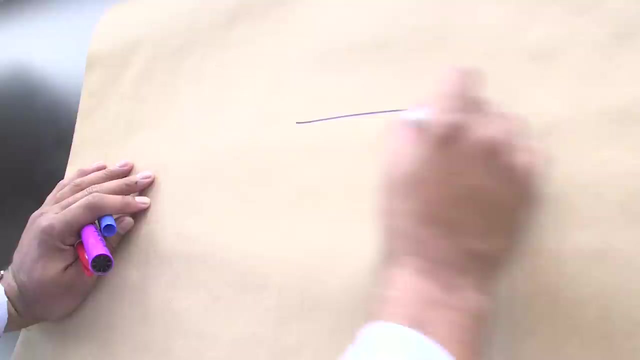 angles on the same side stay with me: less than two right angles, then the two lines, if produced indefinitely, meet on the side which are the angles less than two right angles. It's not catchy, is it? No, There's a lot of words, wordy, And let's see what it means: Two straight lines for. 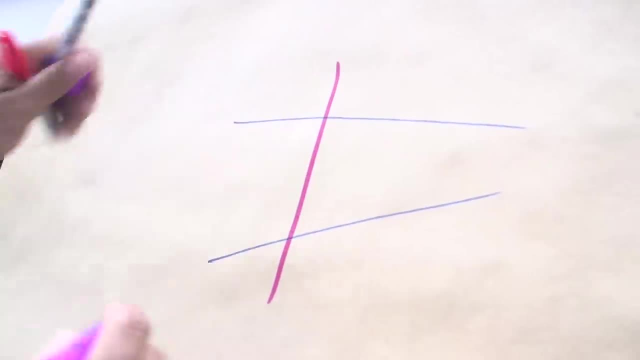 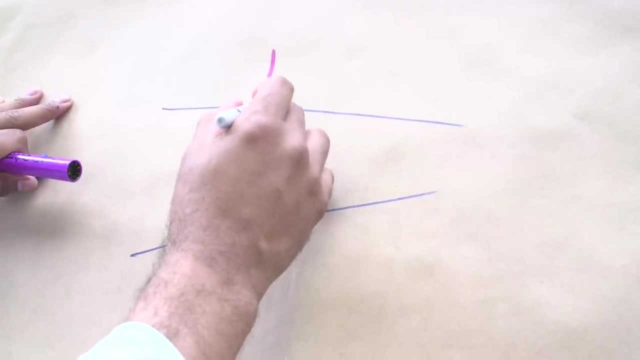 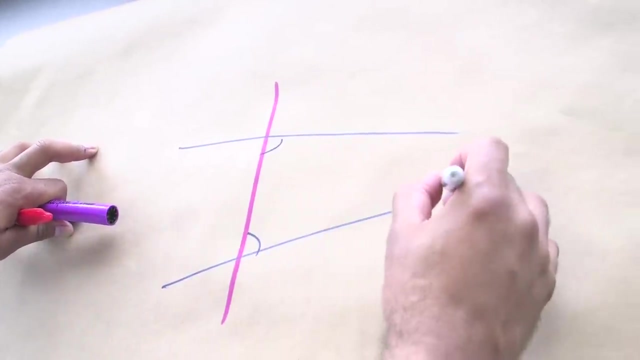 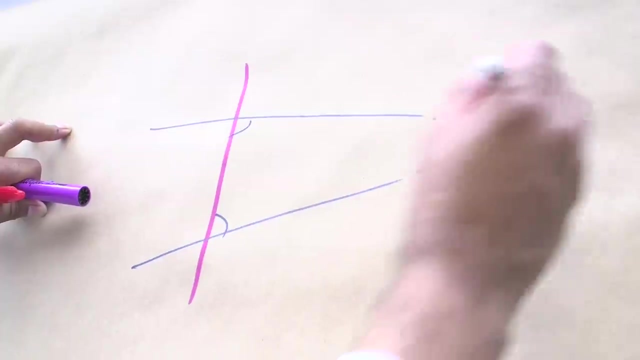 instance, We're going to put a third one, in which lies on top Now the wordy bit about the interior angles being less than two right angles. are those interior angles there? And then the axiom says it is these two straight lines. If these two lines are extended, then there will be a point where they meet. 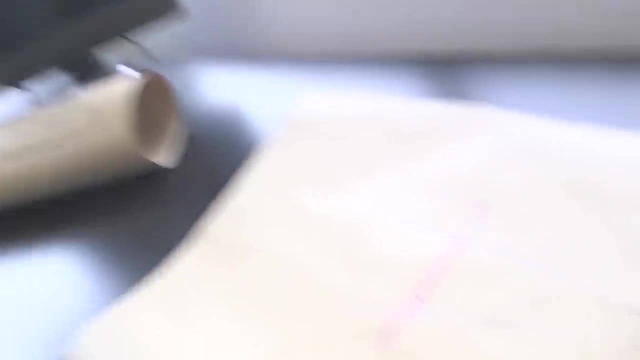 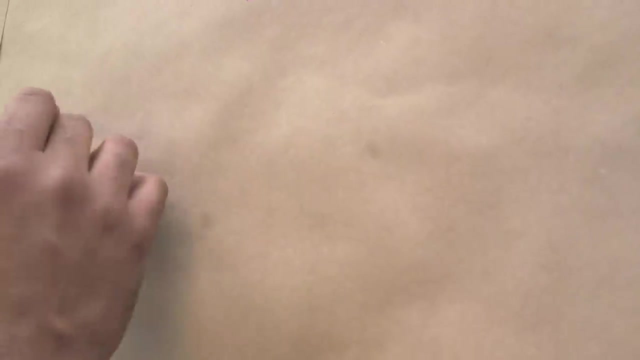 So if these aren't 90, they're going to crash. That's right. An equivalent way of saying this statement is the following: So if you have a line and a point not on that line, let's say here: then there exists a one and 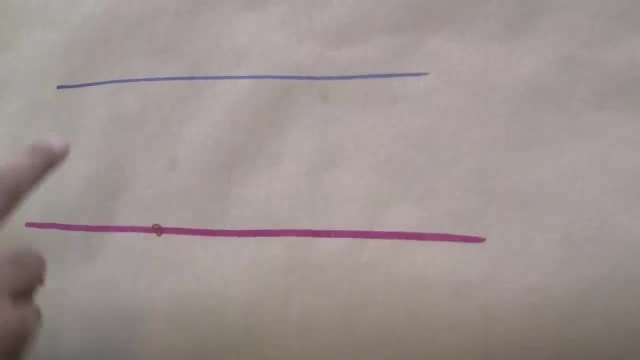 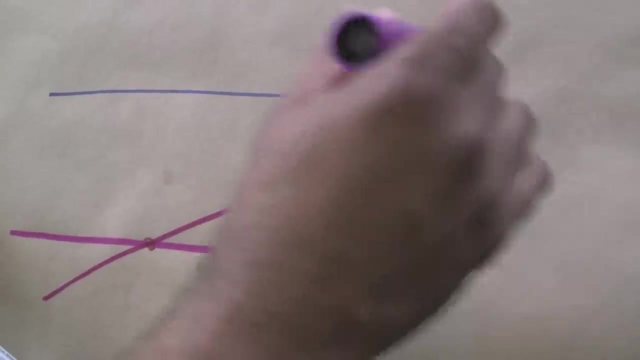 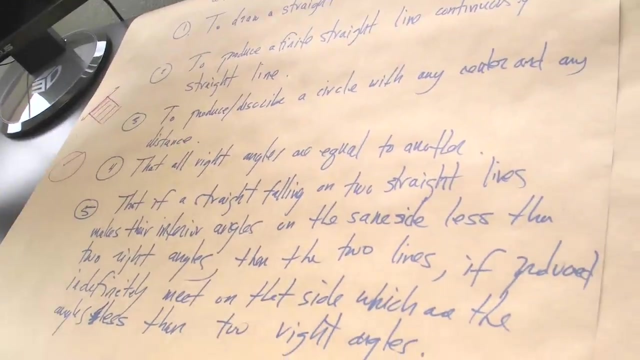 only one line through this point, parallel to the given line. Any other line that we draw Will eventually intersect the given line. So immediately this stands out, This axiom stands out from the others And it's just in its wordiness and the fact that it's not completely straightforward. He was kind of 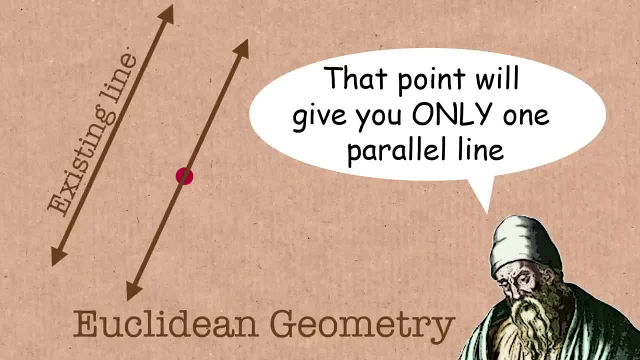 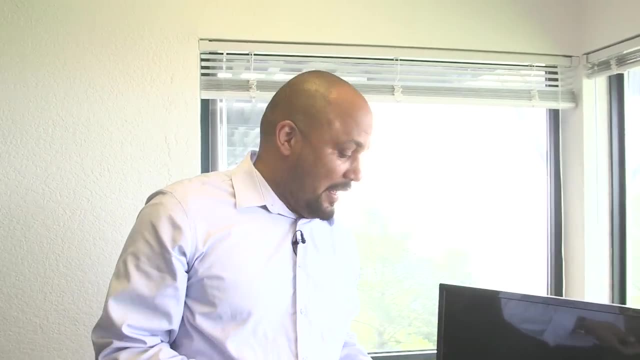 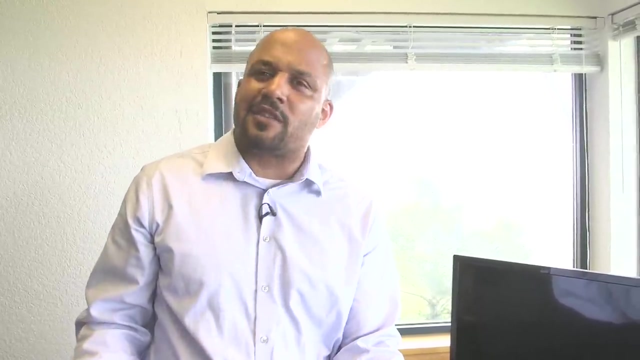 aware of this and that he used it reluctantly And even in the analysis of deducing other propositions and the elements. he waits to use this axiom as long as possible. It's his axiom of last resort. Sure, Yes, And although when we write it down, we can understand why you take it as an axiom, 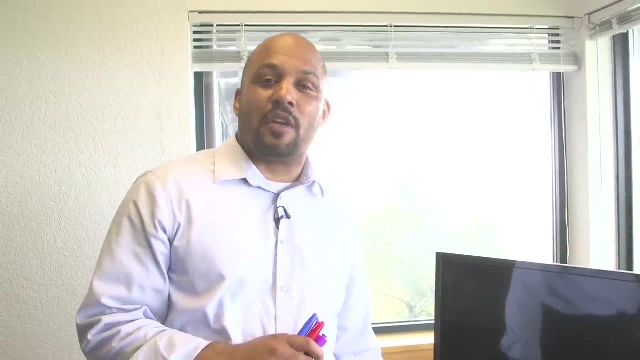 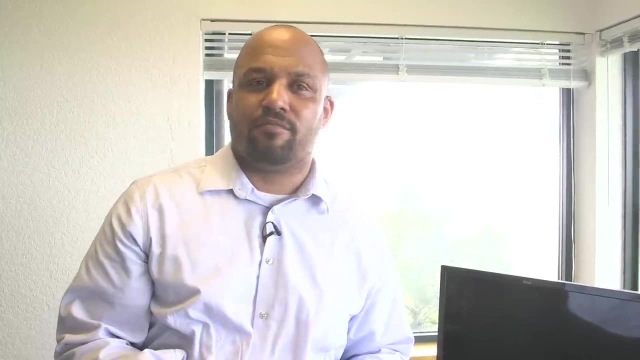 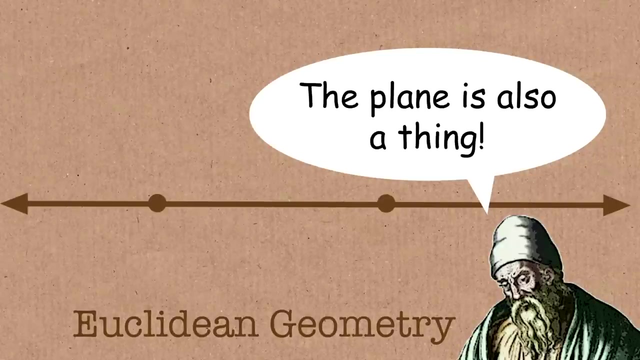 It seems very straightforward, And so here's the amazing story, the 2,000-year-old story of this revolution, this revolutionary idea. The fifth turns out to have this kind of departure into other worlds. The first two had to deal with lines, points and planes, And the third 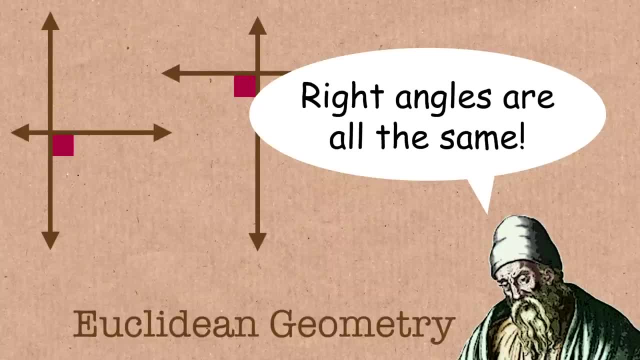 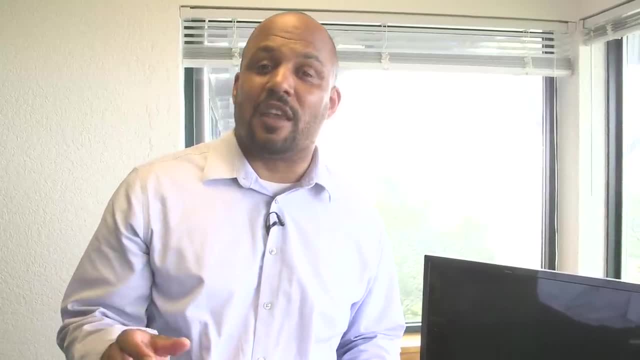 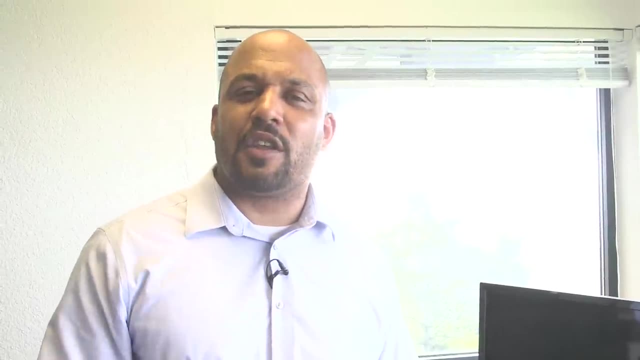 had to do with the… Circles, Circles. Number four is also, there's some more hidden things there. But the fifth, this notion of parallelism, turns out to be the key in kind of unlocking new and mysterious worlds. In 1820, 1830, independently, two mathematicians, a Hungarian Bollai and a 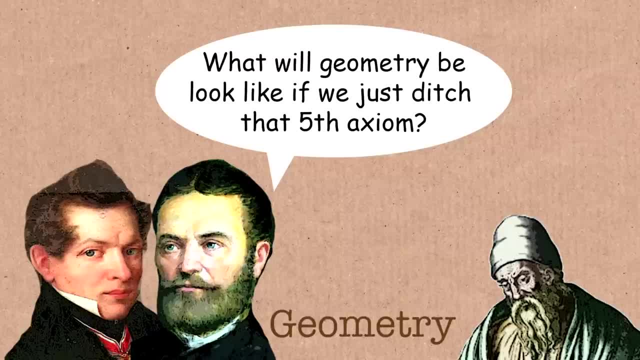 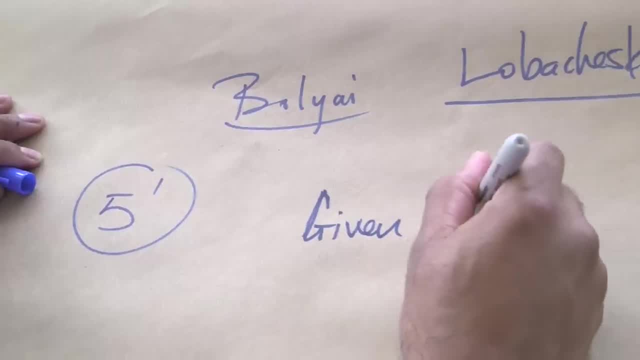 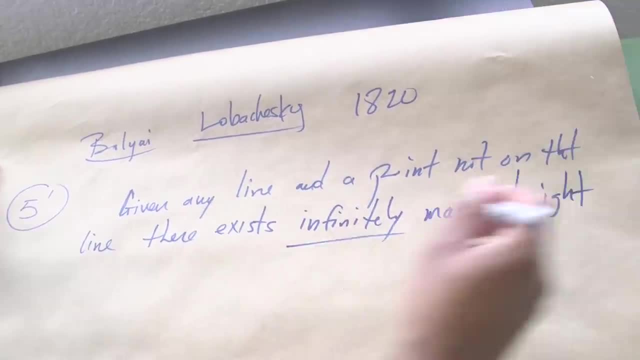 Russian Lobachevsky. they independently discovered what we now call hyperbolic geometry And the fifth axiom. so we can write: maybe… Maybe five prime can be stated like this: Given any line and a point not on that line, there exists infinitely many straight lines through that point, parallel to the given line. 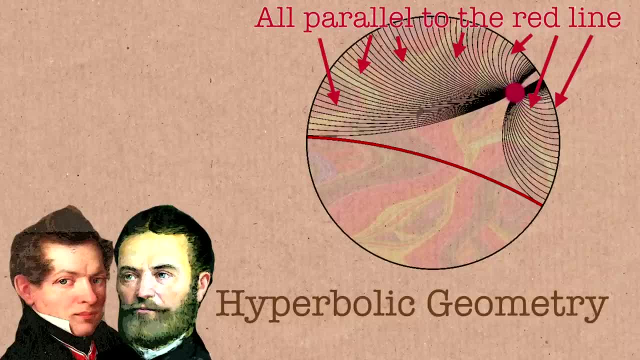 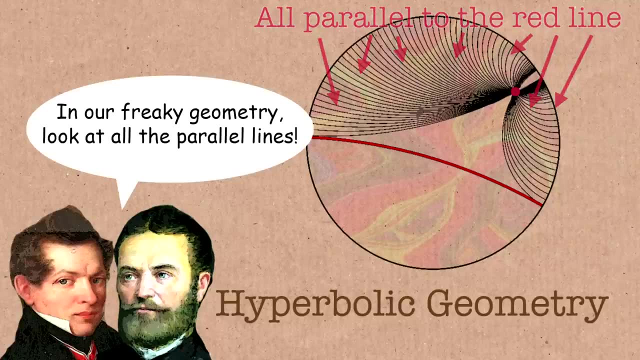 So parallel meaning not intersecting. A moment ago we drew something that showed there was only one parallel line. Now you're saying there are infinite. That's right. Where can these be drawn? What does this look like? So this new world is the hyperbolic plane which they've created? 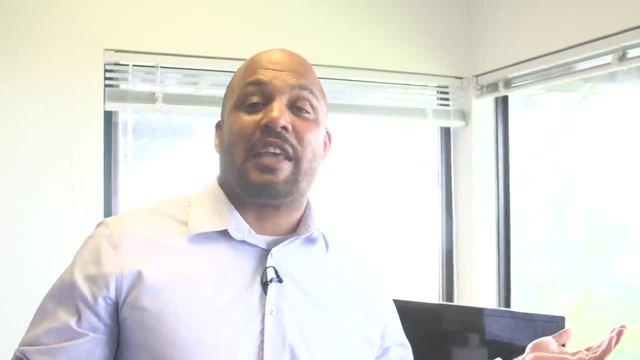 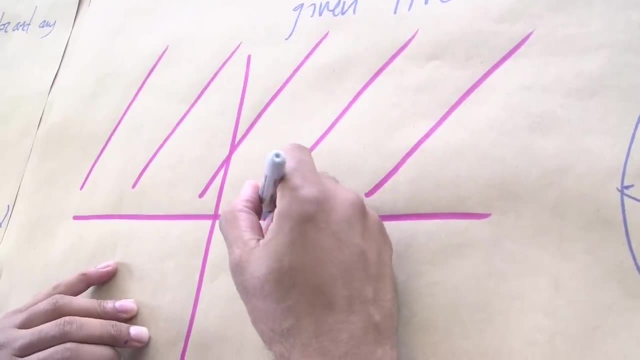 Bollai actually said: out of nothing, I have created an entire world. So now it turns out that straight lines in the hyperbolic plane, in this model of the hyperbolic plane, look like this: Well, Euclidean vertical lines that intersect this boundary at 90 degrees.